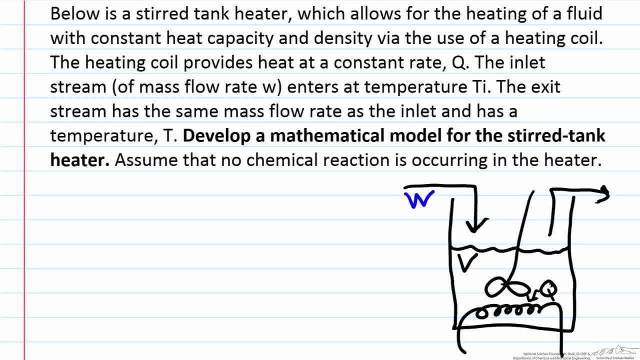 mass flow rate W and an inlet temperature Ti, and exits at that same flow rate W and at temperature T. The fluid is heated by the use of a heating coil, provided at the bottom of the diagram, in which a constant rate of energy of rate Q is provided to the heater. 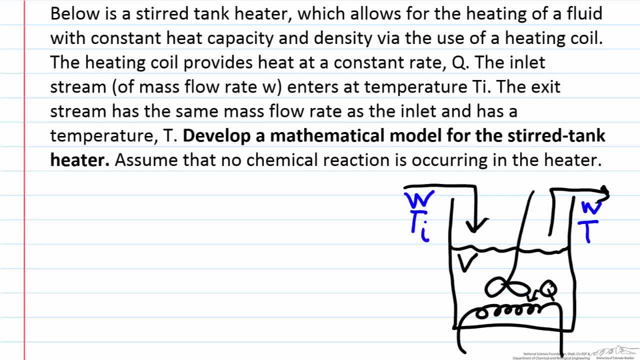 The volume of the liquid inside the stirred tank heater is volume V. So first, before we enter the energy balance, Let's show the fact that the mass balance for this does not really provide much guidance. So if we look at our mass balance first, We recognize the fact that there is no generation. 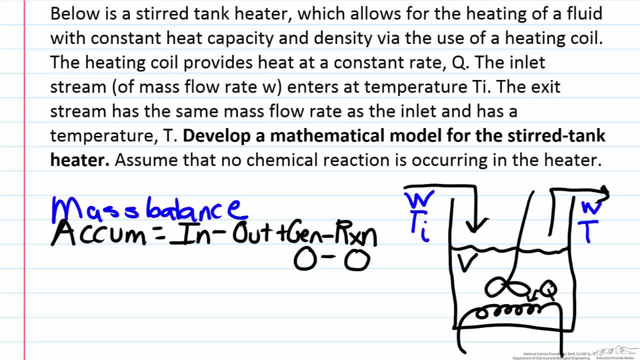 and no reaction going on. if there is no chemical reaction occurring, The inlet flow rate is W and the outlet flow rate is W. So what that means is the fact that the accumulation in this mass balance is zero. So all this is really telling us is that the volume inside 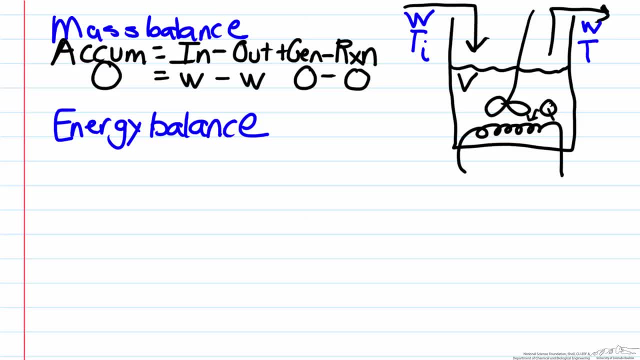 the tank is a constant. So now that we have shown that our mass balance doesn't provide any real fruitful information, We can now go to our energy balance, which is that accumulation of energy equals in minus out Energy in minus energy out plus energy from a chemical reaction. 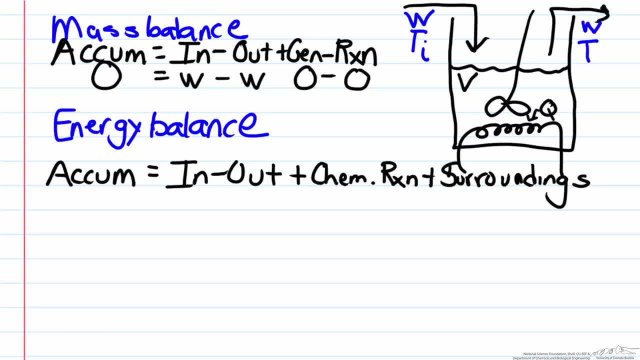 plus energy from the surroundings. An important point to note here is the fact that the sign for the chemical reaction surroundings have been provided here as positive. You have to be very aware of the signs that you are using. So, for example, for an exothermic chemical reaction, the value for this term should be 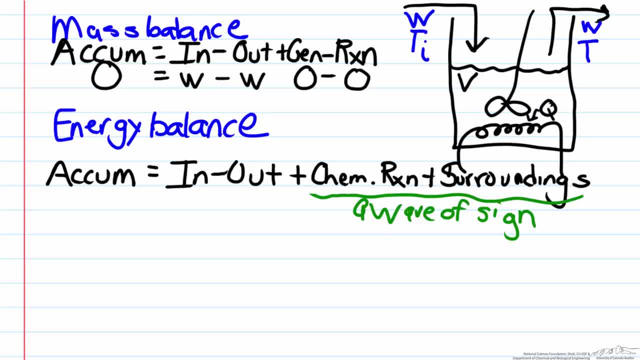 a positive because the temperature of the process inside the system is going to increase. So to begin this energy balance, we'll skip the accumulation term for the time being and we'll focus on the right hand side. The information we have for our interim is the mass flow rate. 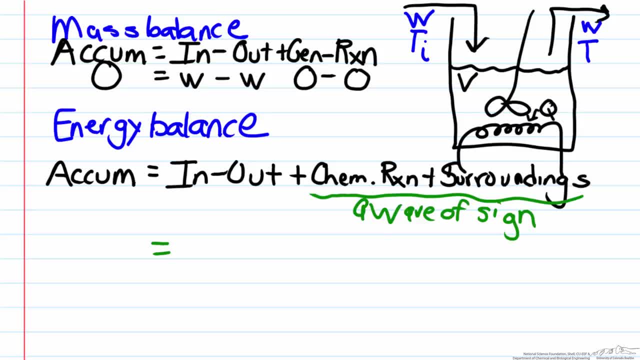 and the temperature. What we need is an energy. So recall from thermodynamics that we can get some idea of an energy per mass. So if we multiply enthalpy, which has units typically of energy, either per mole or per mass, Here we'll go on a per mass basis. And if we multiply it by the mass flow rate, W. 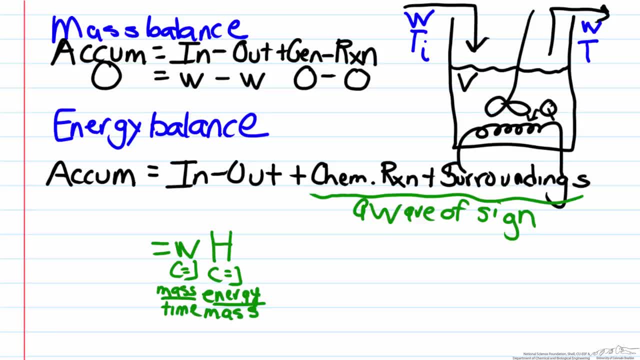 which has units of mass per time. We get our desired units of energy per time. Our interim will be W times the inlet enthalpy of the fluid minus the outlet stream, which is W as a dot, which is double m times W times W. So we get an integral of W plus our energy per 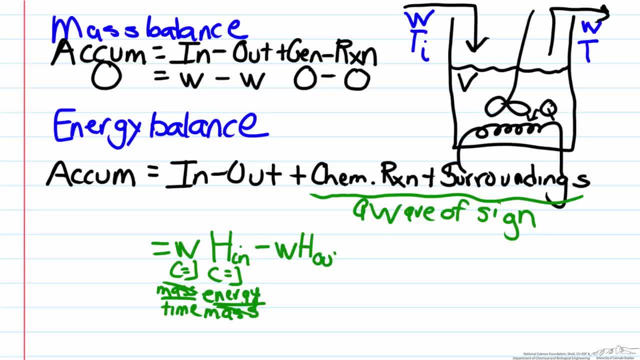 W, now will be times H, out the enthalpy of the exiting stream. there is no chemical reaction going on, so that term goes to zero. and now we have to look at the surroundings term. So our system here has a heating coil which is providing heat at a rate of Q For our 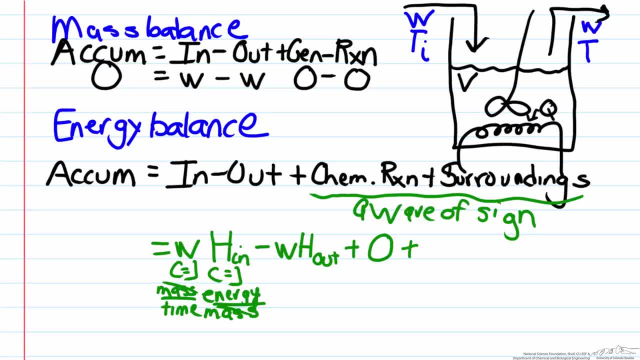 control volume is the inside of the stirred tank heater. this is energy being added to the system. therefore, we are going to want to have this as a plus Q And our accumulation term for now will leave as d energy dt, So d energy dt inside this derivative. what we 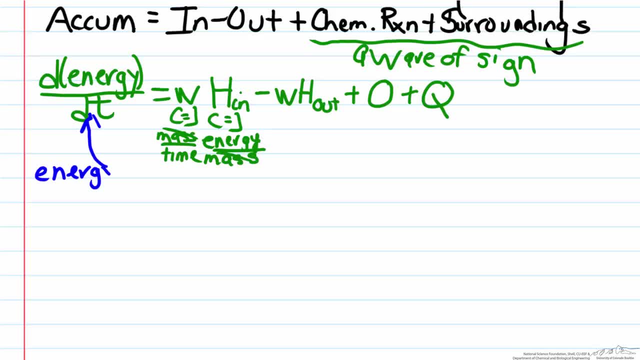 need to find is the amount of energy that is inside the tank that the fluid has. So to determine the energy inside the tank, we actually take a very similar approach to how we handle the inlet and the outlet In the outlet streams, where we are going to be interested in multiplying the mass of. 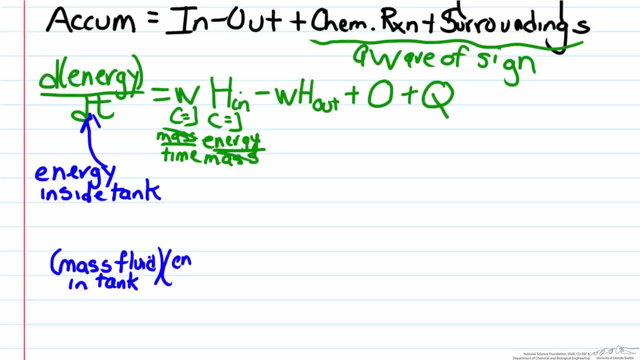 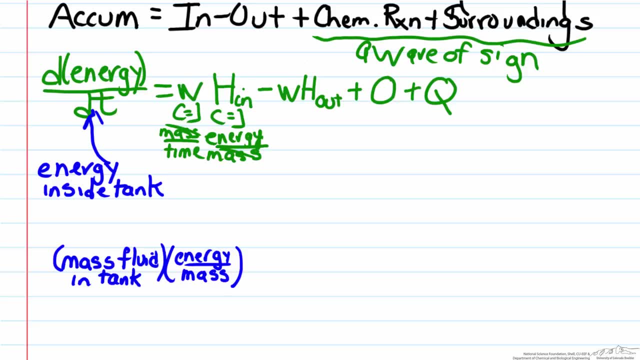 fluid in the tank multiplied by the energy per mass. So first let's find the mass of fluid in the tank. We know the fact that the volume inside the tank of fluid is constant, based on the mass balance at a value of V In order to 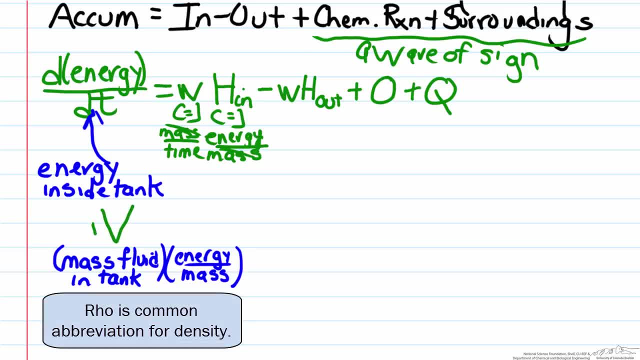 convert from volume to mass. we multiply by rho In order to get the energy per mass. that again is simply the enthalpy, but in this case the enthalpy of the tank, And this will equal the energy term that is in our differential equation. With this information we can restate: 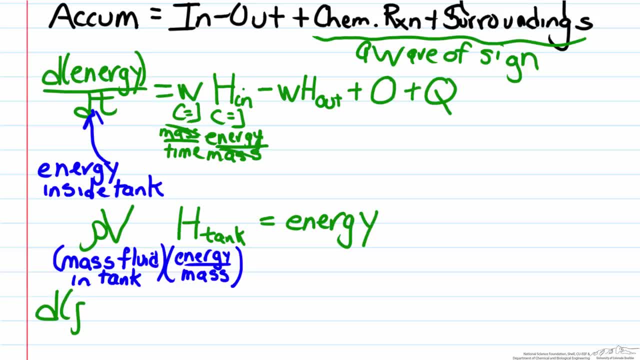 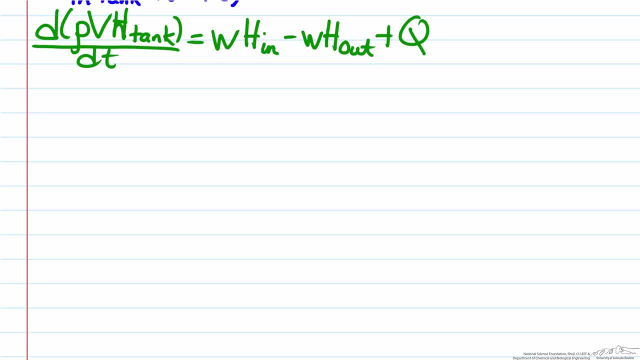 our energy balance. as d rho VH tank dt equals the right hand side From thermodynamics, we can express what the value of the enthalpy is. We can say that for systems with constant heat capacity that H can be expressed as the heat capacity multiplied by the temperature. 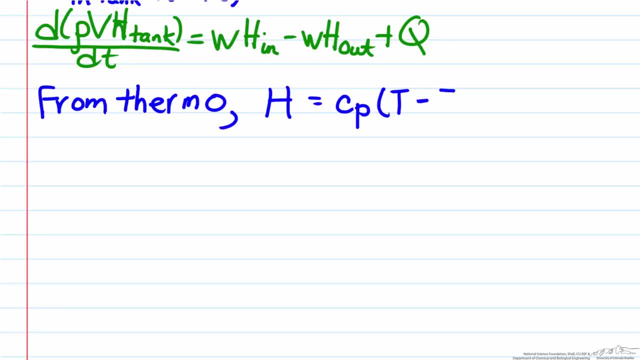 of which the fluid is at minus some reference temperature. And what we will now do is substitute this definition of enthalpy into our energy balance. where enthalpy is located, which is at the tank, the inlet stream and the outlet stream, The derivative will now become rho. 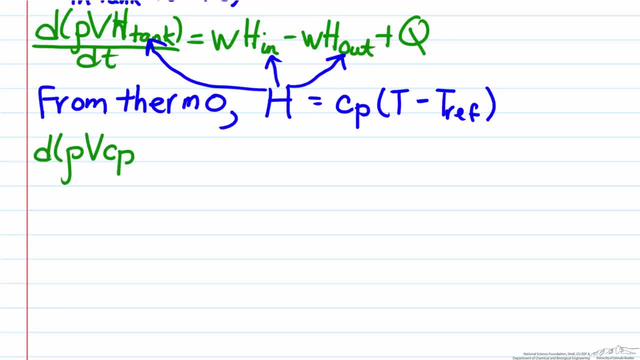 V, Cp times t times t, which is the temperature inside the tank. Since the tank is well mixed, that means the fact that the temperature of the outlet stream of t is identical to the temperature inside the tank. So therefore this will just be t minus t, ref dt. Our in turn becomes W. 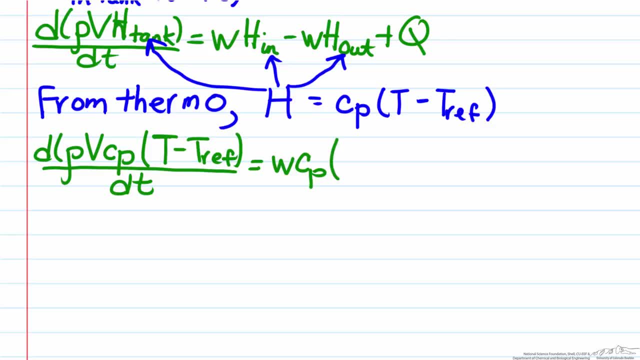 times Cp. Here the inlet stream enters at t i, So it will be t i minus t ref, And this will be t i minus t ref dt. We can do a very similar evaluation for the outlet stream, which is at temperature t, And then we add the q term. We can now take advantage of some simplifications. 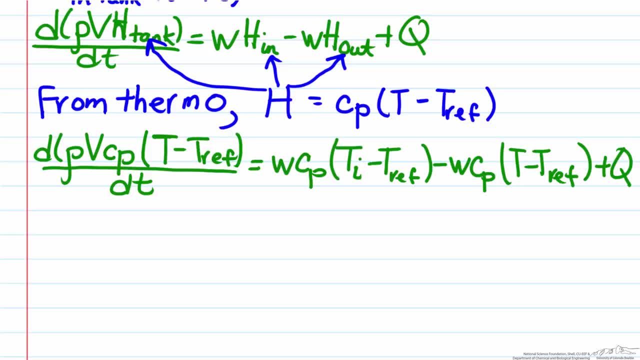 On the left hand side, the reference temperature is a constant value. Therefore, if we take the derivative with respect to time, the value of the t ref part will go to zero. Although d t ref dt goes to zero, d t dt does not term. On the right hand side, we see the fact that we have negative WCP T ref and then 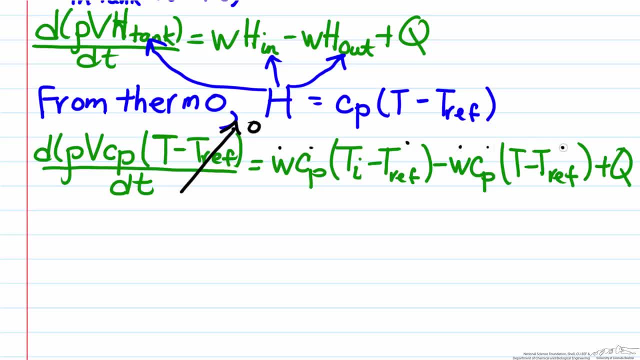 for our second term, we have the same terms, except with an additional minus sign. So, therefore, the T ref terms are going to cancel out an occurrence that is relatively common when doing these energy balances. After these simplifications, we're left with the following, The last step. 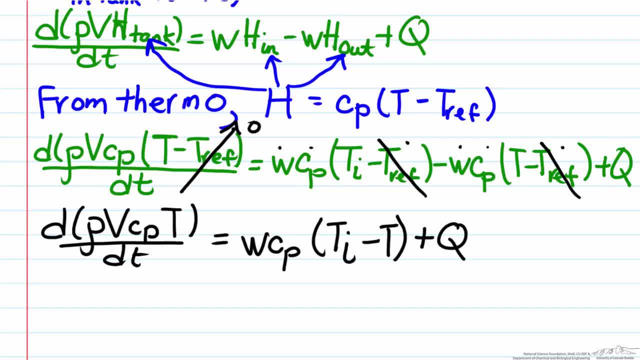 here is to take out a few constants out of the derivative. The problem statement stated that rho and heat capacity were constants and, based on our mass balance, we know that the volume is a constant. So therefore we can take all those out of the derivative to: 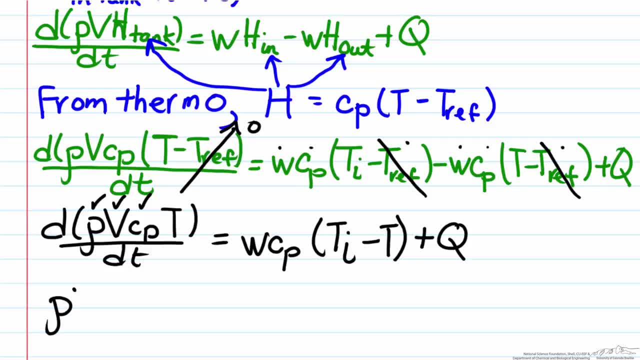 get us to our final answer, which is that rho, VCP dt. dt equals WCP multiplied by the difference between the inlet temperature and the outlet temperature, which is also the tank temperature plus Q. Thank you.